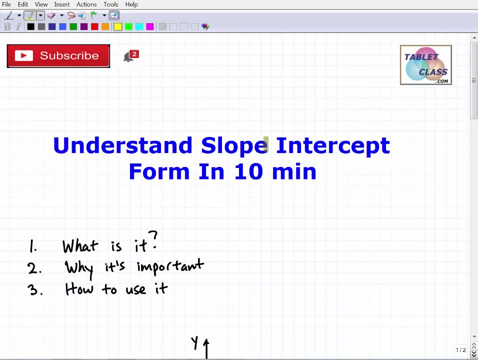 Okay, let's talk about the slope intercept form of a linear equation, And what I want to do is try to really upgrade your knowledge in this area. or maybe it's just going to be a review for you in about 10 minutes or so, So I might go a little bit over, maybe a little bit under, but that's kind of the goal. So if you're new to my videos, I hope you consider subscribing. My background is I'm a math teacher, teach from middle school all the way to college, So I'm going to talk a little bit about the slope intercept form of a linear equation. 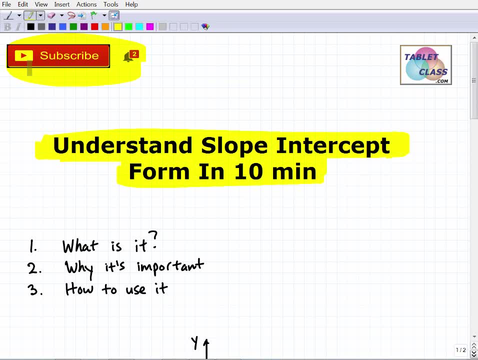 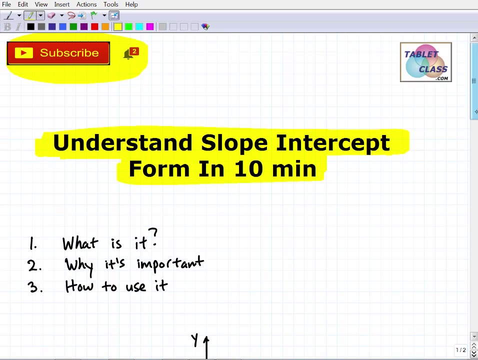 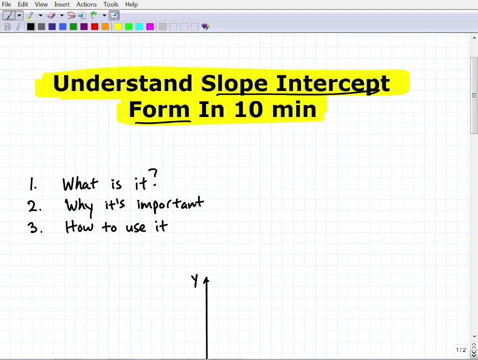 So if you subscribe, I'm posting videos all the time. that will definitely help you for a wide range of math topics, but literally have hundreds and hundreds of videos. If you like my teaching style, then you can have. you know, there's a ton of help on my channel. But with that being said, let's go ahead and cover the three things here, What I want to go over in this video. So slope intercept form. Well, let's talk about, first of all, what is it like, What exactly is it? And then 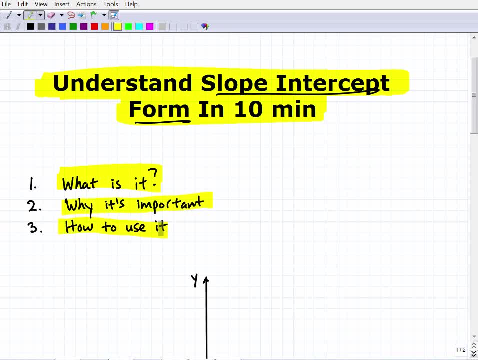 why it's important And then lastly, how to use it. Okay, so if I said here's how to use it and you don't really kind of know what it is or what's important, you know you might know what to like, the mechanics of it, But if you don't know how to apply it or what it's about, then you know you're going to get lost. So let's go ahead and first talk about what it is, Okay. So the slope intercept form is basically this: It's y equals m, x plus b. 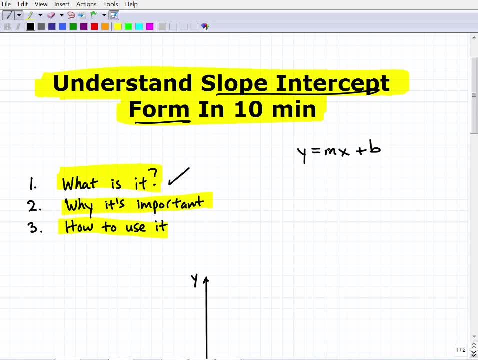 Right. So this is the equation, All right, or the form, Right. what we call a form, it's a general format of a. what of a line? Okay, a line that you graph on x- y axis. So this form here is one type of form that it's that we can read as a format. Okay, we basically can look at it and easily be able to graph lines from it. 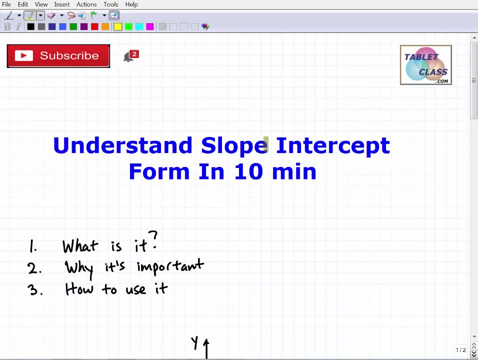 Okay, let's talk about the slope intercept form of a linear equation, And what I want to do is try to really upgrade your knowledge in this area. or maybe it's just going to be a review for you in about 10 minutes or so, So I might go a little bit over, maybe a little bit under, but that's kind of the goal. So if you're new to my videos, I hope you consider subscribing. My background is I'm a math teacher, teach from middle school all the way to college, So I'm going to talk a little bit about the slope intercept form of a linear equation. 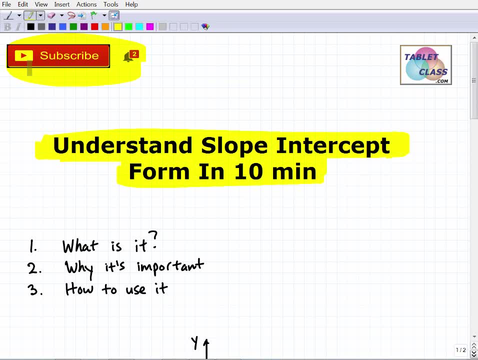 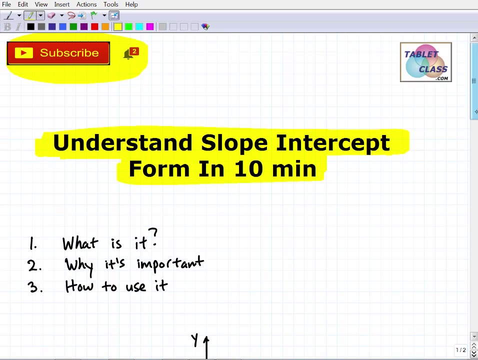 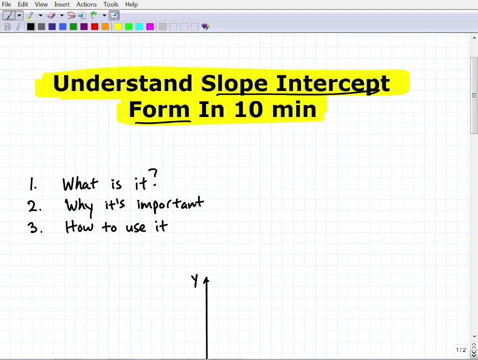 So if you subscribe, I'm posting videos all the time. that will definitely help you for a wide range of math topics, but literally have hundreds and hundreds of videos. If you like my teaching style, then you can have. you know, there's a ton of help on my channel. But with that being said, let's go ahead and cover the three things here, What I want to go over in this video. So slope intercept form. Well, let's talk about, first of all, what is it like, What exactly is it? And then 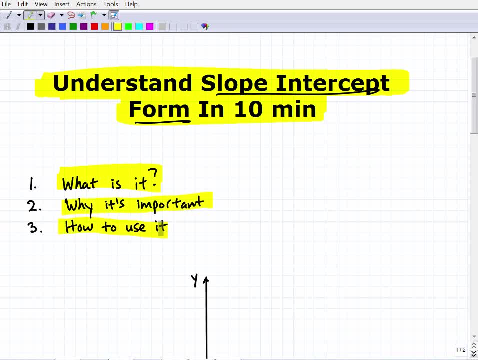 why it's important And then lastly, how to use it. Okay, so if I said here's how to use it and you don't really kind of know what it is or what's important, you know you might know what to like, the mechanics of it, But if you don't know how to apply it or what it's about, then you know you're going to get lost. So let's go ahead and first talk about what it is, Okay. So the slope intercept form is basically this: It's y equals m, x plus b. 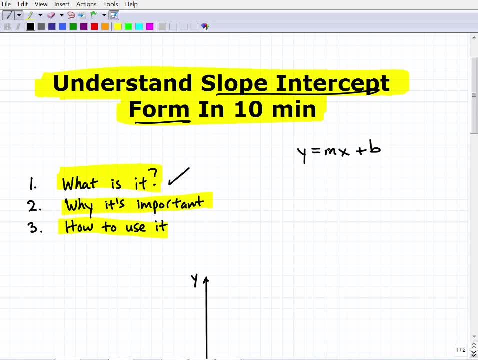 Right. So this is the equation, All right, or the form, Right. what we call a form, it's a general format of a. what of a line? Okay, a line that you graph on x- y axis. So this form here is one type of form that it's that we can read as a format. Okay, we basically can look at it and easily be able to graph lines from it. 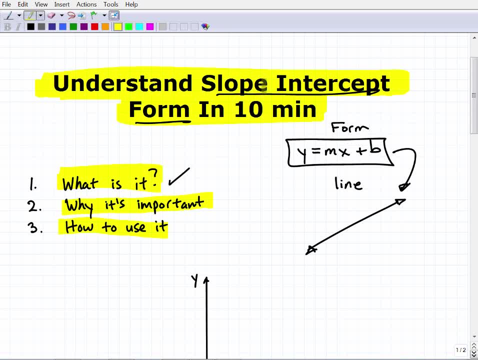 Okay now, why is that the case? Well, let's just look at the, the name of what we're talking about. It's a slope intercept. So where's the slope part? Well, the m is the slope part And the b here is the intercept. And the intercept we're talking about is the y intercept. Okay, so, kind of getting a little bit ahead of myself, But this is basically what it is. It's a form that we can see lines. So this is the form that we can see lines. 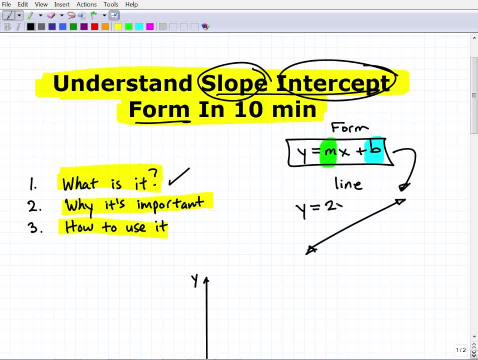 So this is the general form, But if I saw a line like this: y equals two x plus one, this particular line is written in this particular format. there's just one y, there's a number in front of the x, which is the slope, and then there's some of the number over here to the to the right of that, And that is going to be our intercept information. So with this we can graph lines. Okay, extremely important fundamental skill in algebra must know how to do it. And when it comes to 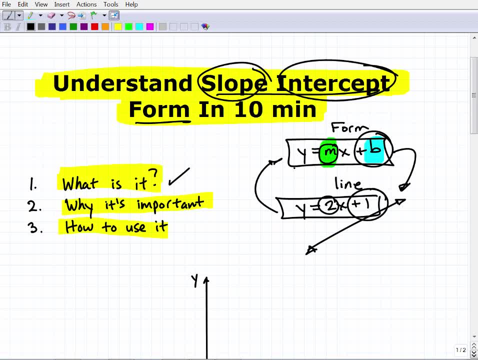 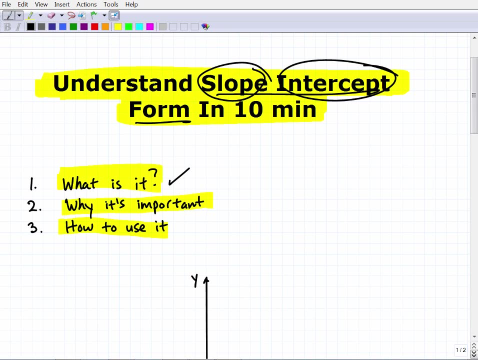 linear equations or lines, equations of lines. this is the most common. this is extremely, extremely important to to get. So if you stick with me, you're going to understand this Alright. so that's what it is Now kind of already answered. the second thing: why it's? why it's important? Well, it's important because this is one of the most common ways that we use to graph lines. So when lines are written like 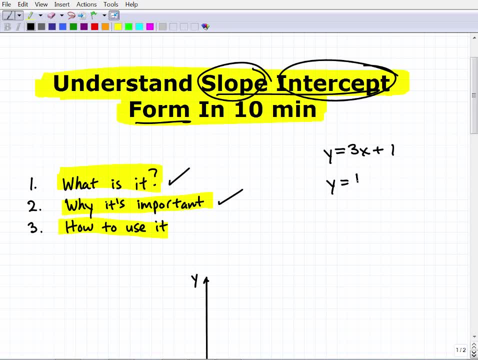 in this form here. alright, I'm just kind of showing you examples. All these lines here are in slope intercept form. Okay, Now I call these lines, but technically they're called linear equations, And that's just an equation of a line, Alright, so we get some sort of line on the x- y axis. These equations express this line, define that line. Okay, and the slope intercept form is the most common. Now, oftentimes, 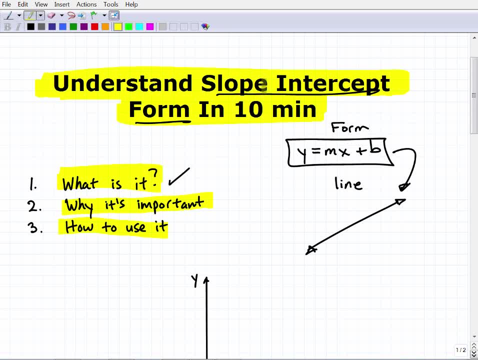 Okay now, why is that the case? Well, let's just look at the, the name of what we're talking about. It's a slope intercept. So where's the slope part? Well, the m is the slope part And the b here is the intercept. And the intercept we're talking about is the y intercept. Okay, so, kind of getting a little bit ahead of myself, But this is basically what it is. It's a form that we can see lines. So this is the form that we can see lines. 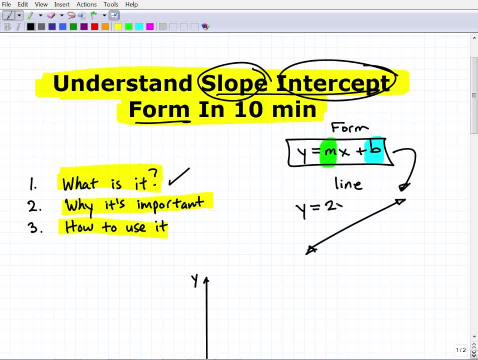 So this is the general form, But if I saw a line like this: y equals two x plus one, this particular line is written in this particular format. there's just one y, there's a number in front of the x, which is the slope, and then there's some of the number over here to the to the right of that, And that is going to be our intercept information. So with this we can graph lines. Okay, extremely important fundamental skill in algebra must know how to do it. And when it comes to 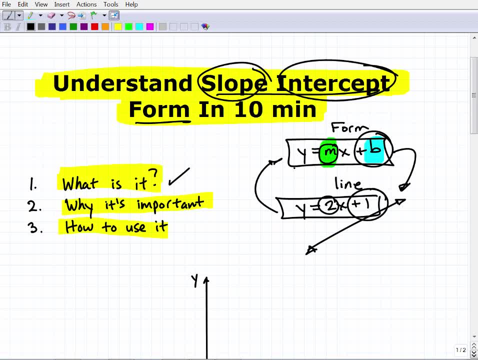 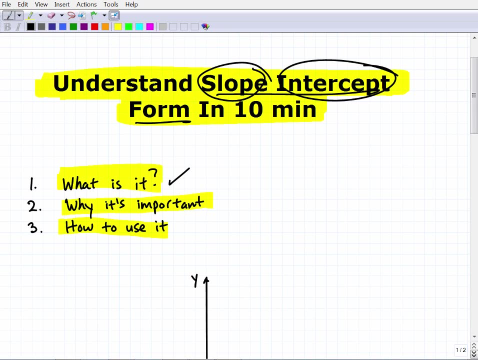 linear equations or lines, equations of lines. this is the most common. this is extremely, extremely important to to get. So if you stick with me, you're going to understand this Alright. so that's what it is Now kind of already answered. the second thing: why it's? why it's important? Well, it's important because this is one of the most common ways that we use to graph lines. So when lines are written like 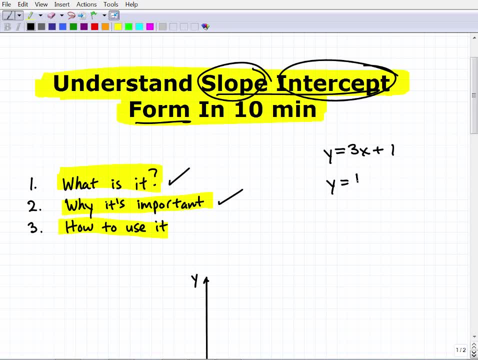 in this form here. alright, I'm just kind of showing you examples. All these lines here are in slope intercept form. Okay, Now I call these lines, but technically they're called linear equations, And that's just an equation of a line, Alright, so we get some sort of line on the x- y axis. These equations express this line, define that line. Okay, and the slope intercept form is the most common. Now, oftentimes, 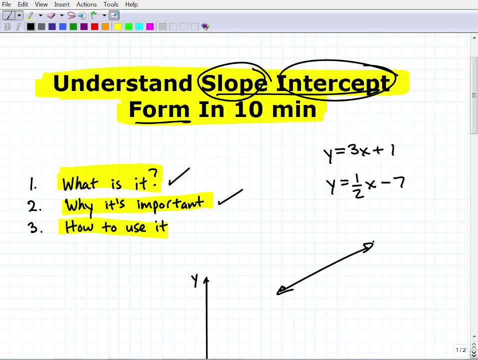 later, after you master this, you're going to get to a part of your math course where it's going to say: hey, what's the equation of a line if a line has a slope of two thirds and it has a intercept of seven? Okay, now you're going to be given information about a line And what they want is the equation to that line And specifically, what they're going to be looking for is to give you that equation, most generally in that slope intercept form. 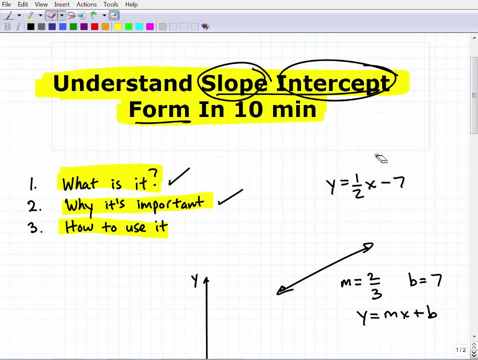 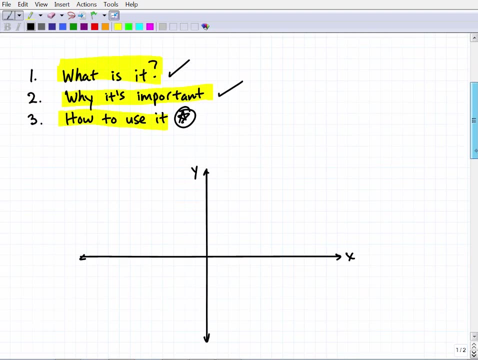 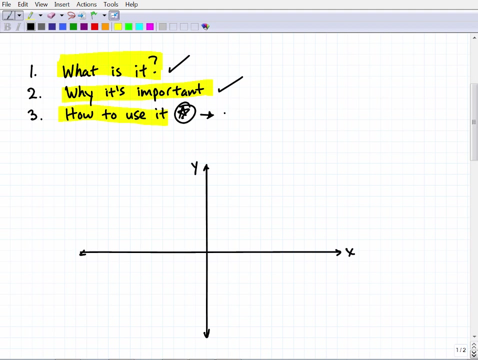 Okay, again, slope intercept form the most common way to express lines in algebra. Alright, so let's get down to this last fun part here: how to use it. So let's go through a couple basic examples Now. you might get a little- hopefully you won't get a little lost on this. I'm gonna make it as clear as I can, But you may have to review the slope of a line. I have a. 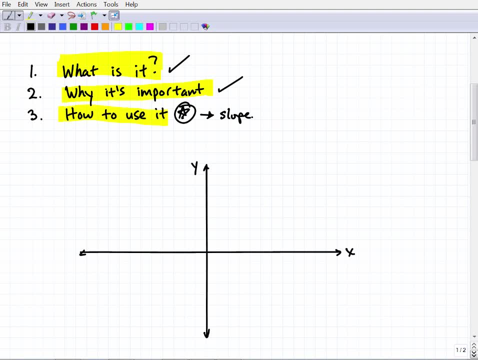 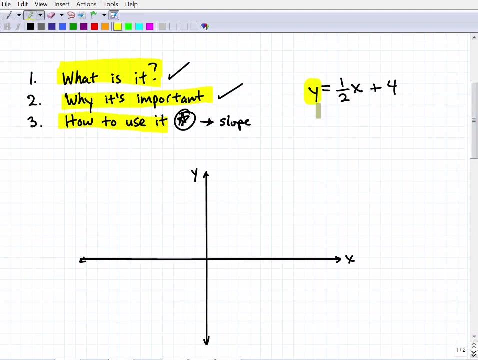 videos on that as well, But I'll explain that in here in a second. Okay, so let's get a basic example. Let's say I have y equals one half plus four. whoops, one half x plus four. Now this line is in slope intercept form. Why? Because we have one y, we have some sort of number in front of an x And then we have another number. 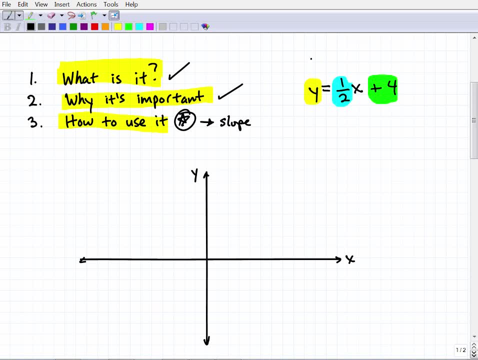 over here, plus or minus off to the right. now, the form, the general form, the algebraic form of the slope intercept is: y equals m, x plus B. so the number in front of the X, this number here is the slope information, this is the slope okay which we refer to as the variable M, and then this number, this plus or minus. 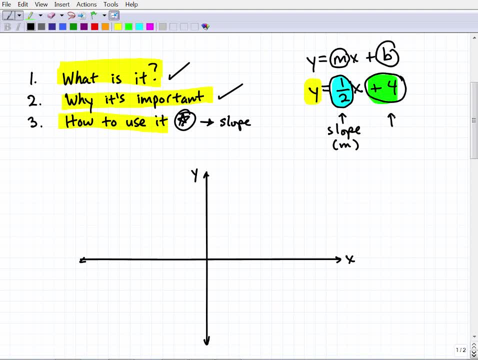 number over here. this B is the intercept, but specifically it's the Y intercept, okay. so the way we're going to do this is, when you're graphing lines using the slope intercept form, you always start. it's kind of my: put a little set of directions here. you always start with the B, okay, or the Y intercept, okay. this. 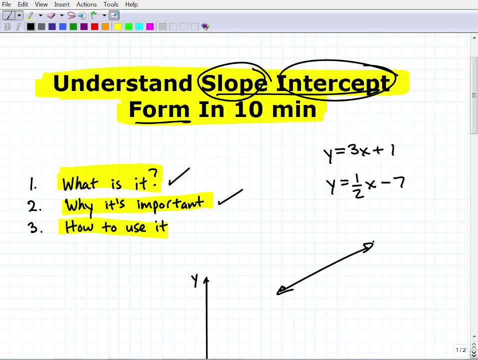 later, after you master this, you're going to get to a part of your math course where it's going to say: hey, what's the equation of a line if a line has a slope of two thirds and it has a intercept of seven? Okay, now you're going to be given information about a line And what they want is the equation to that line And specifically, what they're going to be looking for is to give you that equation, most generally in that slope intercept form. 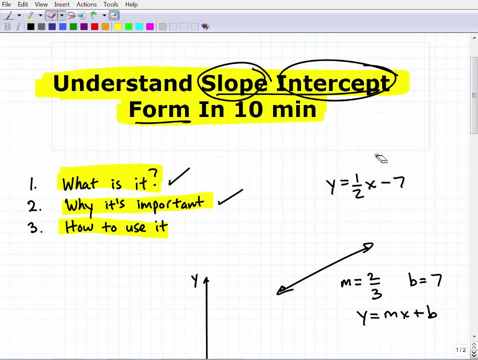 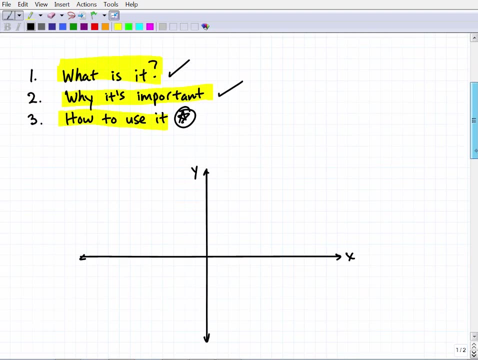 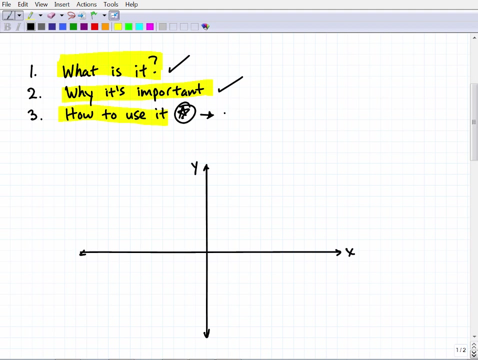 Okay, again, slope intercept form the most common way to express lines in algebra. Alright, so let's get down to this last fun part here: how to use it. So let's go through a couple basic examples Now. you might get a little- hopefully you won't get a little lost on this. I'm gonna make it as clear as I can, But you may have to review the slope of a line. I have a. 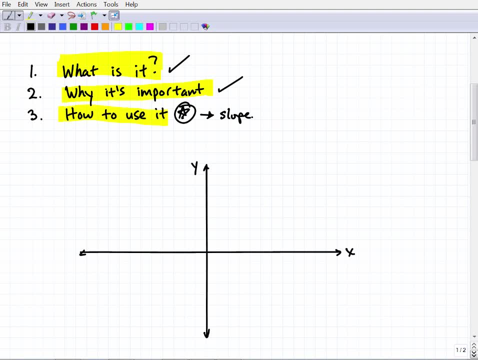 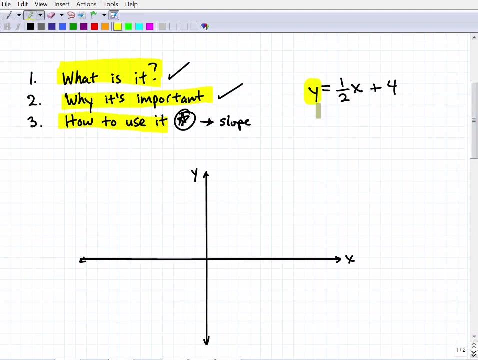 videos on that as well, But I'll explain that in here in a second. Okay, so let's get a basic example. Let's say I have y equals one half plus four. oops, one half x plus four. Now this line is in slope intercept form. Why? Because we have one y, we have some sort of number in front of an x And then we have another number. 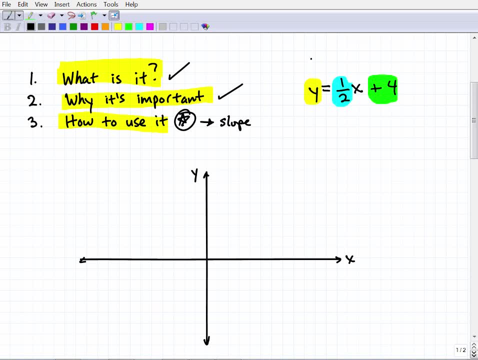 over here, plus or minus off to the right. now, the form, the general form, the algebraic form of the slope intercept is: y equals m, x plus B. so the number in front of the X, this number here is the slope information, this is the slope okay which we refer to as the variable M, and then this number, this plus or minus. 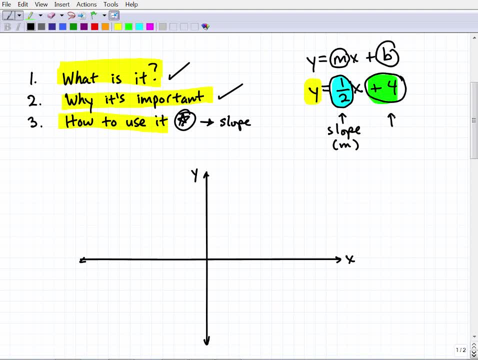 number over here. this B is the intercept, but specifically it's the Y intercept, okay. so the way we're going to do this is, when you're graphing lines using the slope intercept form, you always start. it's kind of my: put a little set of directions here. you always start with the B, okay, or the Y intercept, okay. this. 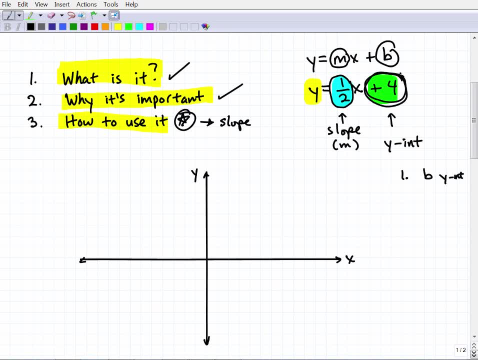 is where we start. so here I have four. all right, so I go to my little XY chart here. and now you're saying: okay, Y, intercept, what is that? well, here you do. we see the y-axis. right, this is the y-axis, this is the vertical one. so this line is going to chop through it or intercept it at four. 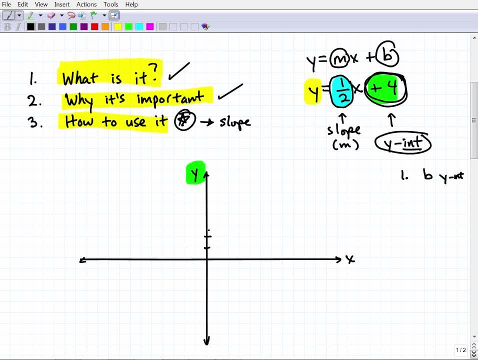 so we just count up the y-axis one, two, three, four, that's it. so we put a little, just a little point there, and this is one point that's on the line. now, if I have a line here or any line, I'm going to put a little point on the line and 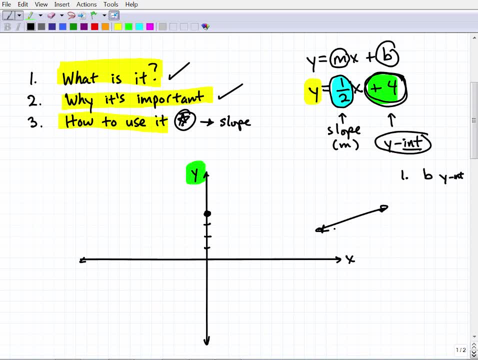 any line. how many points do I need to actually graph it? well, I need a one point and I need at least another point. right? if I have two points, I can draw a line through those two points and I will have graphed the line. so this is the. 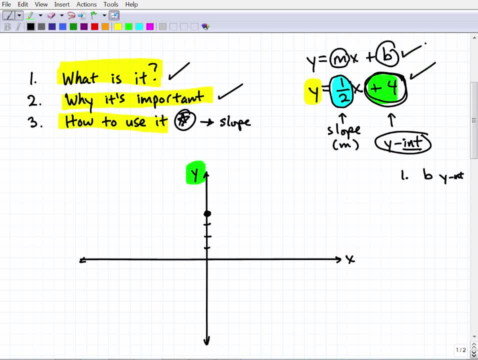 idea here. so when we start off with the B information or the y intercept information, this gives us one point. let me go ahead and just write it here, all right. so this gives us our first point, our first point. that's going to be on a line now to get to the second point. 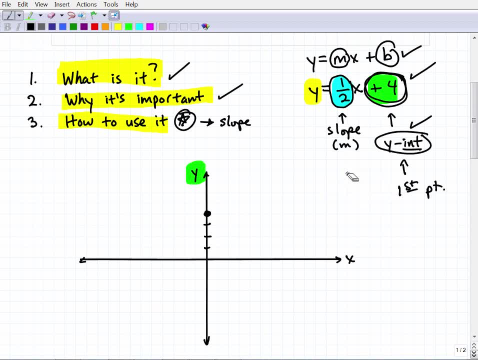 we have to use the slope information, so this is a little bit where students get a little bit confused. so the slope here is M is equal to 1 half right, that's the slope. so think of the slope as kind of like a set of driving directions to get. 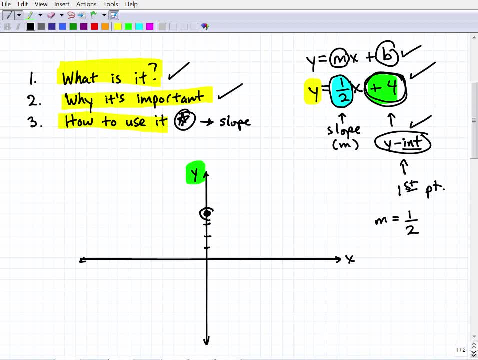 to your second point. so we're going to be leaving here, this place, and we're going to be using the slope information as a set of driving directions to get to our second point. let's say it's over here. once I get to that second point, I 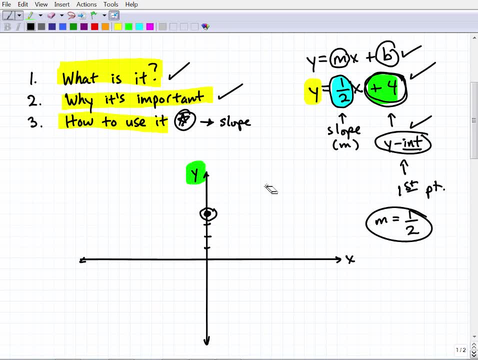 can draw my line right. I just need two points. so how does this work? so let me write this here: M equals 1 half, and then we'll finish this problem up. so the slope, by definition, is the rise over the run of a line. now, basically the way that's. 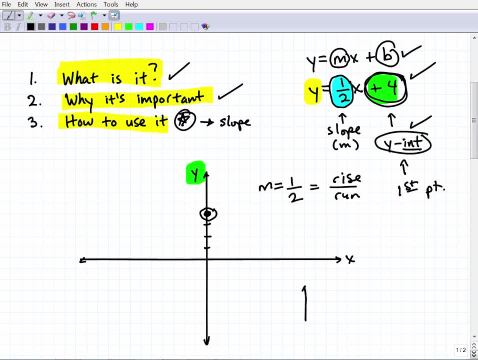 going to look is this: you're going to either go up and then to the right, so your driving directions are either going to be up and to the right, so it's going to be up and to the right, or down and to the right. okay, so if your slope is, 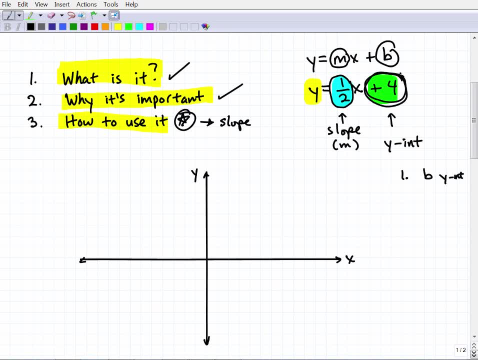 is where we start. so here I have four. all right, so I go to my little XY chart here. and now you're saying: okay, Y, intercept, what is that? well, here you do. we see the y-axis. right, this is the y-axis, this is the vertical one. so this line is going to chop through it or intercept it at four. 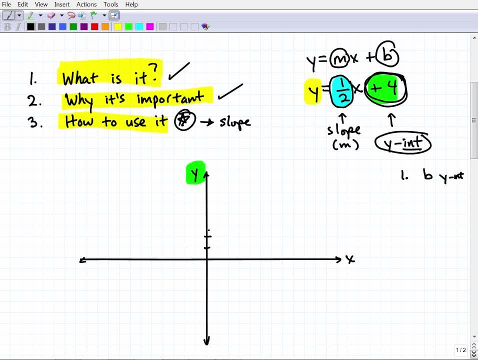 so we just count up the y-axis one, two, three, four, that's it. so we put a little, just a little point there, and this is one point that's on the line. now, if I have a line here or any line, I'm going to put a little point on the line and 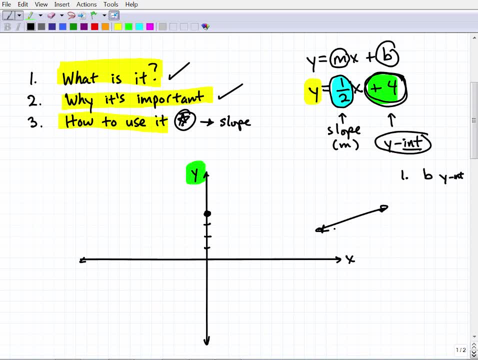 any line. how many points do I need to actually graph it? well, I need a one point and I need at least another point. right? if I have two points, I can draw a line through those two points and I will have graphed the line. so this is the. 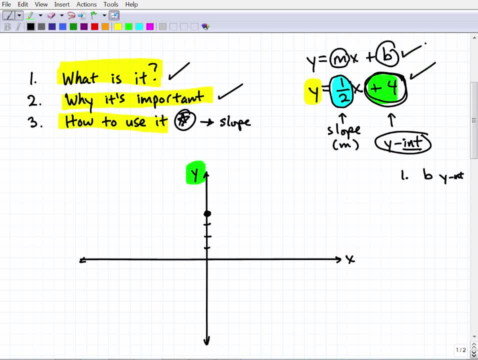 idea here. so when we start off with the B information or the y intercept information, this gives us one point. let me go ahead and just write it here, all right. so this gives us our first point, our first point. that's going to be on a line now to get to the second point. 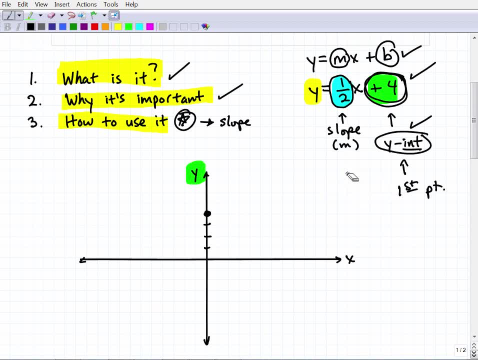 we have to use the slope information, so this is a little bit where students get a little bit confused. so the slope here is M is equal to 1 half right, that's the slope. so think of the slope as kind of like a set of driving directions to get. 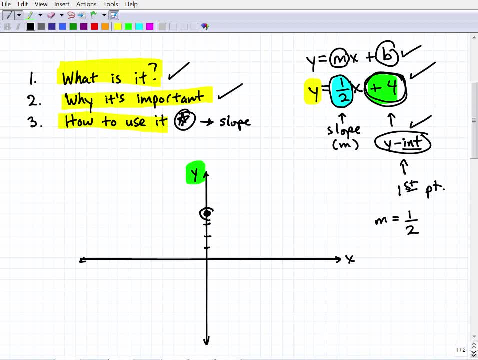 to your second point. so we're going to be leaving here, this place, and we're going to be using the slope information as a set of driving directions to get to our second point. let's say it's over here. once I get to that second point, I 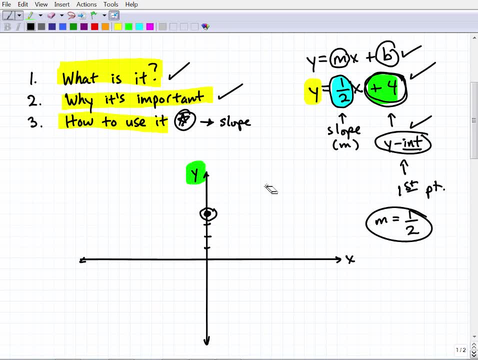 can draw my line right. I just need two points. so how does this work? so let me write this here: M equals 1 half, and then we'll finish this problem up. so the slope, by definition, is the rise over the run of a line. now, basically the way that's. 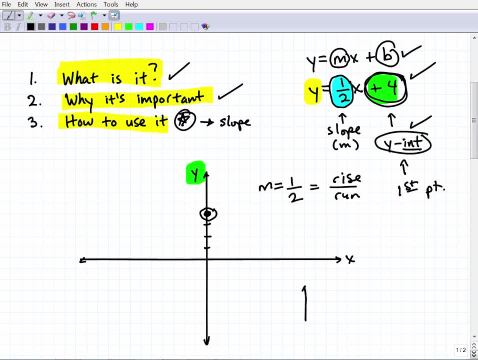 going to look is this: you're going to either go up and then to the right, so your driving directions are either going to be up and to the right, so it's going to be up and to the right, or down and to the right. okay, so if your slope is, 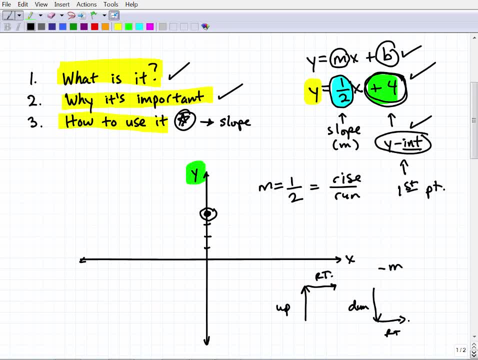 negative. if you have a negative slope, you're going to go down and to the right, and if your slope is positive, you're going to go up and to the right, okay. so your rise is how much you go up or down, okay, and your run is how much you go off. 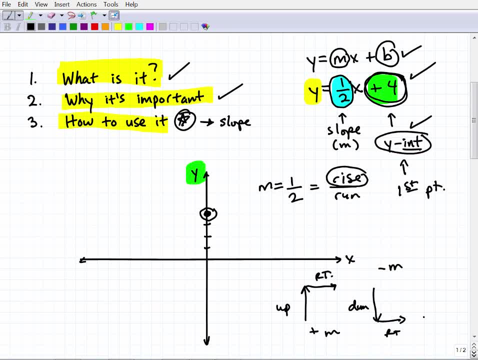 to the right. So if we understand that, let's take this point here, this particular example, and we'll go through it. So m is equal to 1 half. so my rise is 1.. So from my first point, my y-intercept, not from the origin, from my first point I'm going to go up 1.. 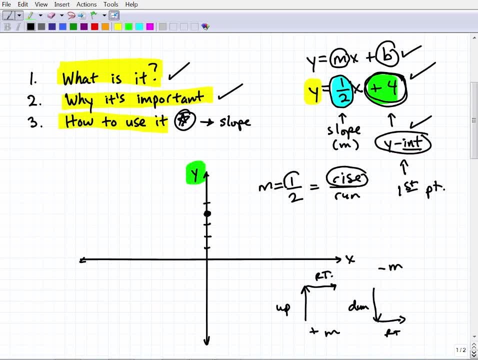 Do you see that? So I'm leaving my first point. I'm going up 1.. So I went up 1.. Now remember I told you it's either up and to the right or down and to the right. So once I've done that, now I look at this run information. 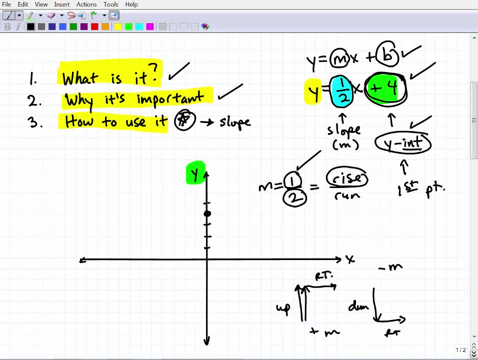 So I'm going to make a right-hand turn from that. first when I went up 1, now I'm going to go out 1,, 2.. And there is my second point. That's my second point there. So now that I have that, I can just go ahead. let me erase this real quick and just draw my line. 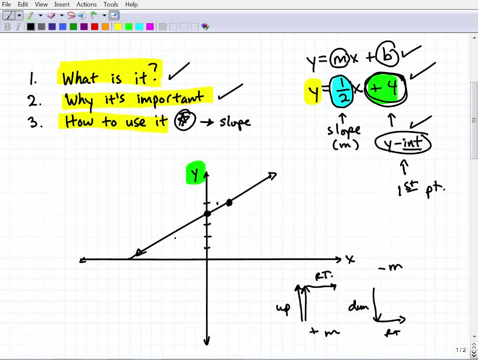 And there it is. So this is the line of the equation: y equals 1 half x plus 4.. Okay, y equals 1 half x plus 4.. That linear equation is written in slope-intercept form, and we used that form to easily graph this line. 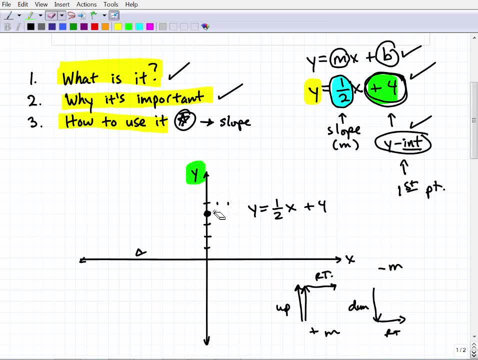 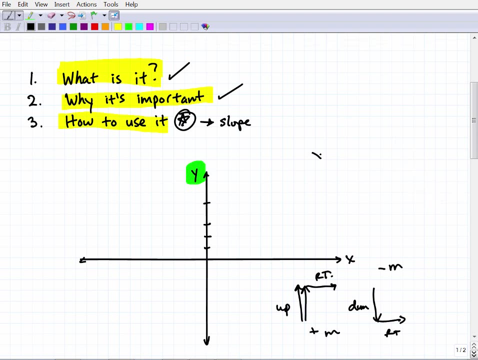 Okay, let's do one real quick example, because I don't want to make this video too long, But let's do another one, okay? So if you understand everything or like everything I just said, you know, then hey, you got it okay. 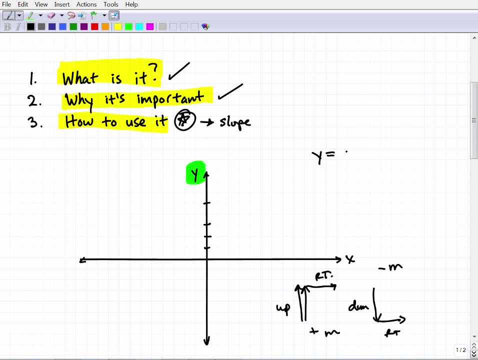 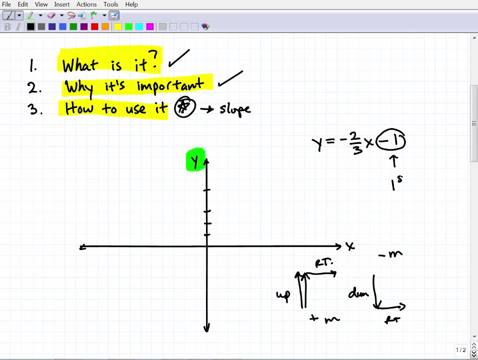 We don't have to make this stuff more complicated than it is. So let's use: y equals negative 2 thirds x minus 1, okay, All right, so we're going to start here with our y-intercept. This is going to be our first point, right? 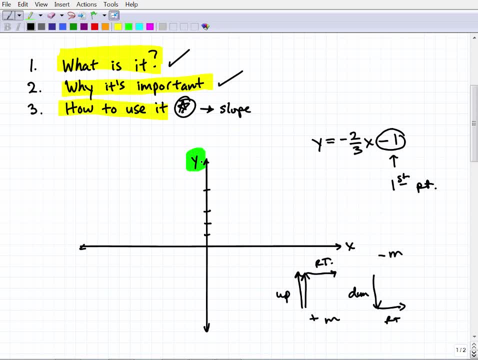 So our first point. So where do I go? Well, I'm going to look on the y-axis. I'm going to go down 1, so it's right here That's negative 1,. okay, So that's done. 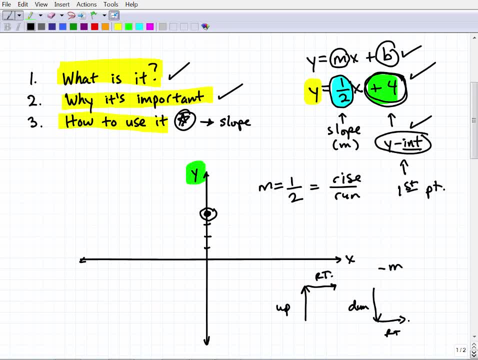 negative. if you have a negative slope, you're going to go down and to the right, and if your slope is positive, you're going to go up and to the right, okay. so your rise is how much you go up or down, okay, and your run is how much you go off. 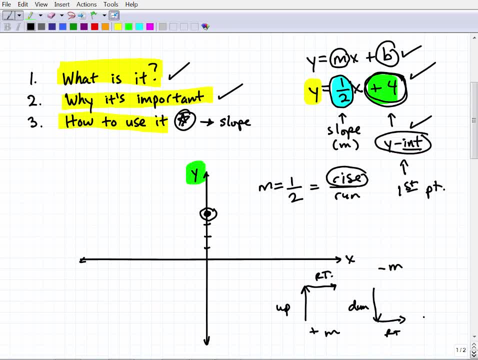 to the right. so if we understand that, let's take this point here, okay, this particular example, and we'll go through it. okay, so M is equal to 1 half. so my rise is 1. so from my, my first point, my y-intercept, not from the origin, from my first point, I'm 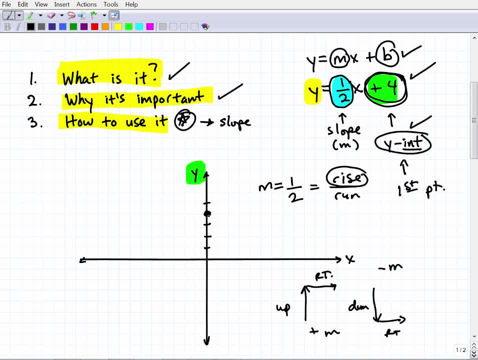 going to go up 1. do you see that? so I'm leaving my first point. I'm going up 1, all right, so I went up 1. now, remember I told you it's either up and to the right or down and to the right. so once I've done that, 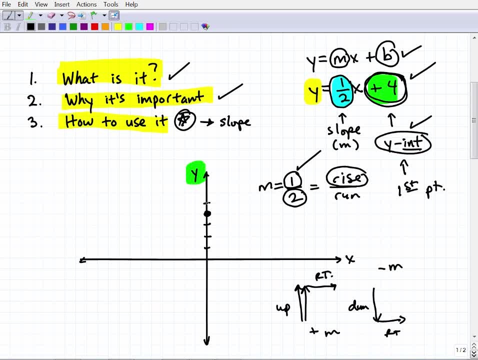 look at this run information. so I'm going to make a right-hand turn from that. first when I went up 1, now I'm going to go out 1, 2 and there is my second point. okay, that's my second point there. so now that I have that, I can just 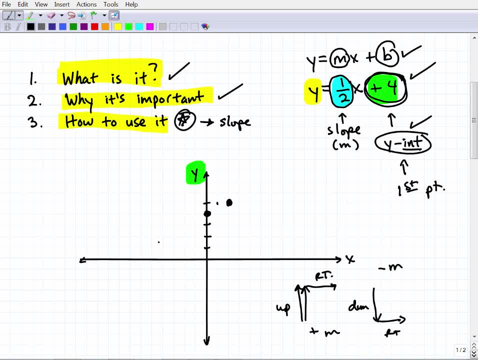 go ahead and erase this real quick and just draw my line. okay, and there it is. okay. so this is the line of the equation: y equals 1 half x plus 4. okay, y equals 1 half x plus 4. that linear equation is written in slope. 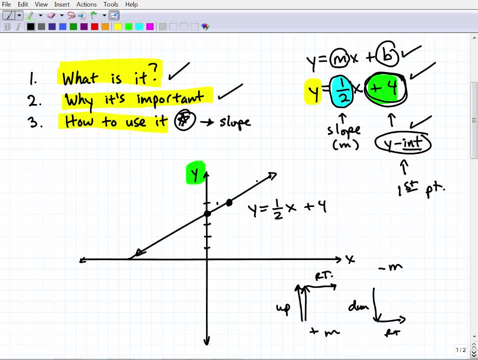 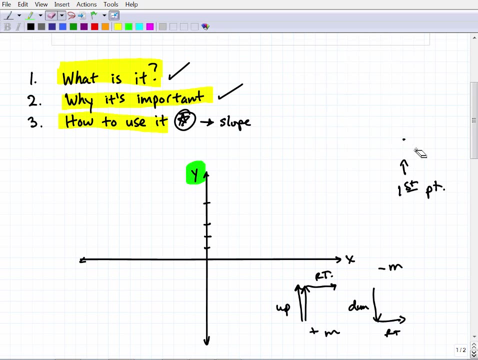 intercept form and we used that form to easily graph this line. okay, let's do one real quick example, because I want to make this video too long, but let's do another one, okay, so if you understand everything, I like everything I just said, you know, then hey, you got it, okay it. 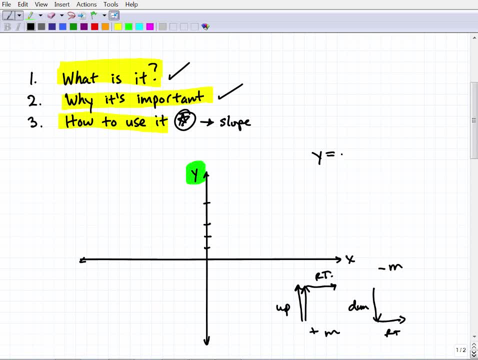 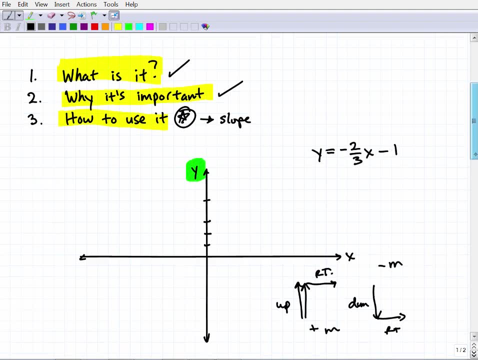 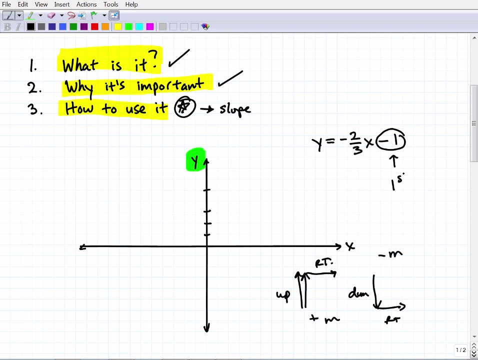 we don't have to make this stuff more complicated than it is, so let's use: y equals negative 2 thirds x minus 1. okay, all right, so we're going to start here with our y-intercept. this is going to be our first point, right? so our first point. 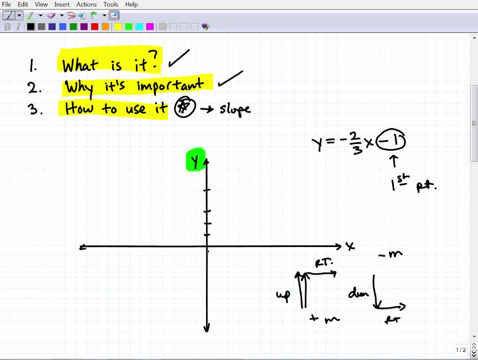 so where do I go? well, I'm going to look on the y-axis. I'm going to go down one. so it's right, here that's negative 1. okay, so that's done. now I'm going to use this slope information to figure out from that point. 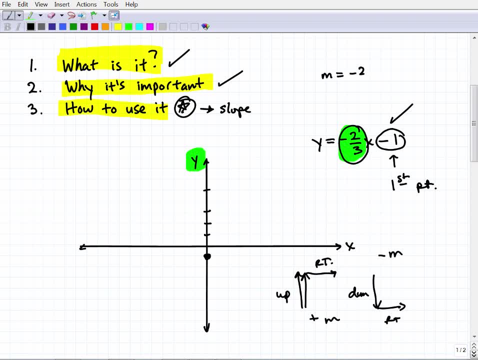 how to get to my second point. so my M is equal to negative 2 thirds. so I told you, when you have a negative slope it's going to be down and to the right. so it's going to be down 2. okay, because your rise is 2, which is negative 2, and 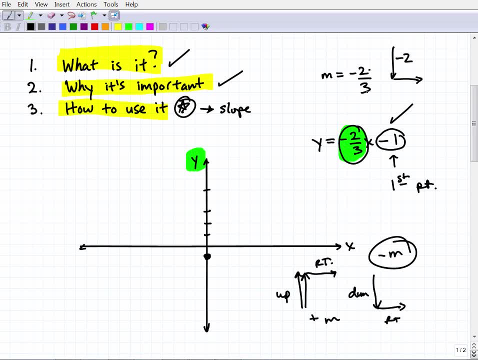 your run, your, your run is always your bottom number on your fraction here. so your run is 3. so from this point I'm going to go down to 1- 2 in the negative direction, and then I'm going to the right: 3. 1, 2, 3 and there's my second. 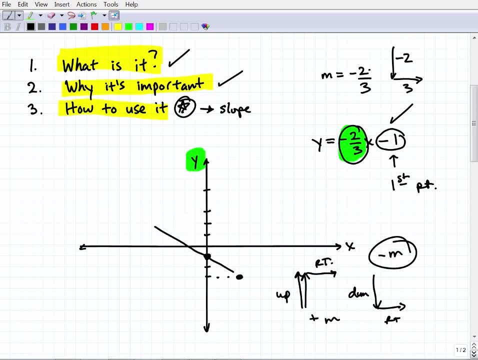 point. and then I just go and draw my nice little tool line through those two points and I graphed the linear equation: y equals negative 2 thirds x minus 1. again, this is a linear equation, it's in intercept form and we love this form because this information, the way this, 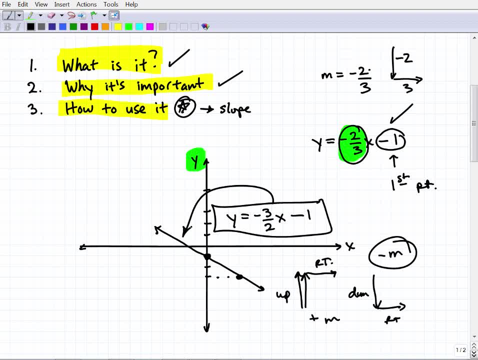 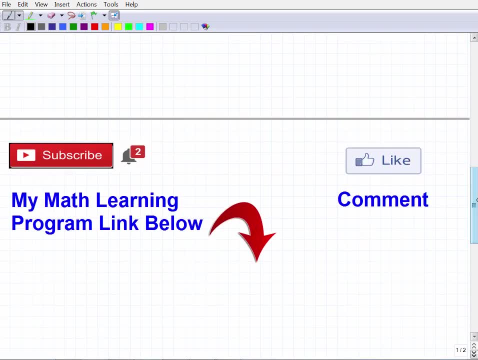 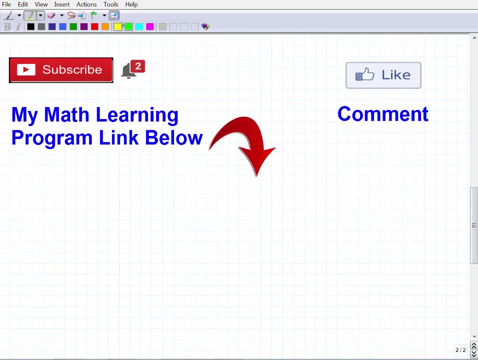 format is it's easy to graph this line. okay, so that's basically it again. we could do a lot more examples. actually have plenty more examples on mind, a lot of my videos, so if you want to check those out, you can't, so hopefully you'll consider subscribing. I also have a complete, many, many full. 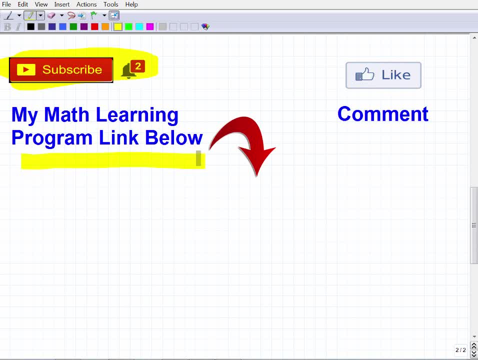 comprehensive math courses. I'll leave a link in the description of this video if you want to check those out. so if you're taking algebra 1, I actually have complete comprehensive algebra 1 programs. I mean I'm talking about full programs where I'm teaching complete lessons going over literally in my 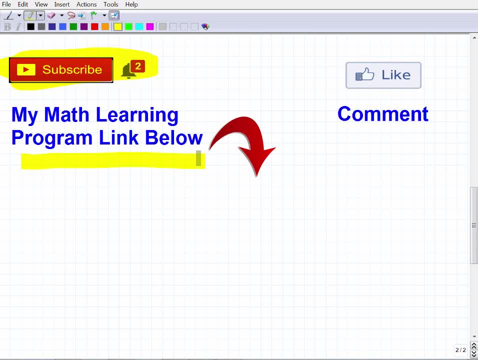 algebra courses, for example, several thousand problems. I'm showing you how to do them step by step, so it's a pretty. it's one of the most comprehensive courses we're learning math learning programs out there. so if you like my teaching style and you really really want to learn from me, then 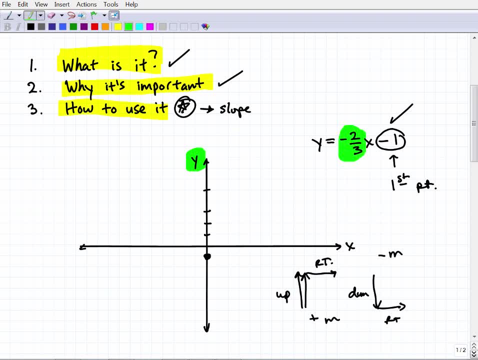 Now I'm going to use this slope information to figure out from that point how to get to my second point. So my m is equal to negative 2 thirds. So I told you, when you have a negative slope it's going to be down and to the right. 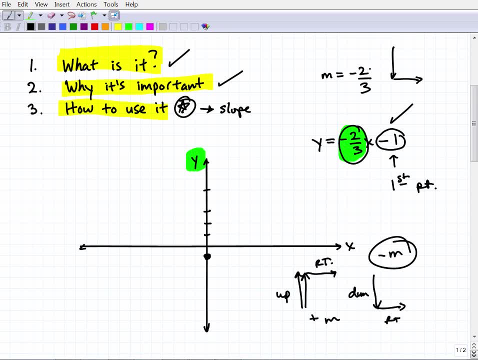 So it's going to be down 2, okay, because your rise is 2.. It's going to be negative: 2. Run: your run is always your bottom number on your fraction here, So your run is 3.. So from this point I'm going to go down to 1,, 2 in the negative direction. 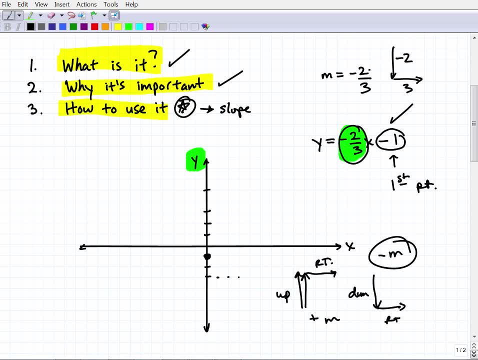 and then I'm going to the right: 3, 1,, 2,, 3, and there's my second point. And then I just go and draw my nice little line through those two points and I graphed the linear equation: y equals negative 2 thirds x minus 1.. 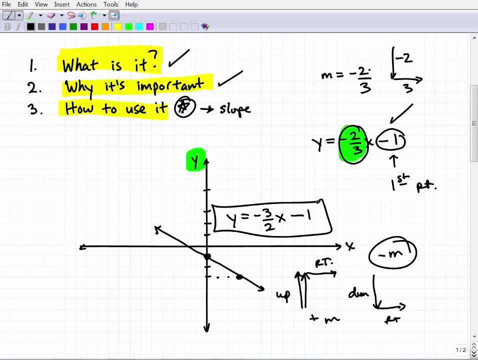 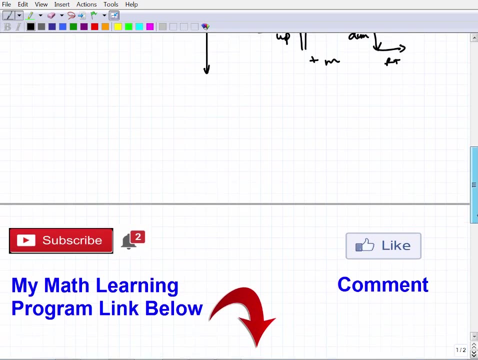 Again, this is a linear equation. It's in slope-intercept form and we love this form because this information, the way this format is, it's easy to graph this line. Okay, so that's basically it. Again, we could do a lot more examples. 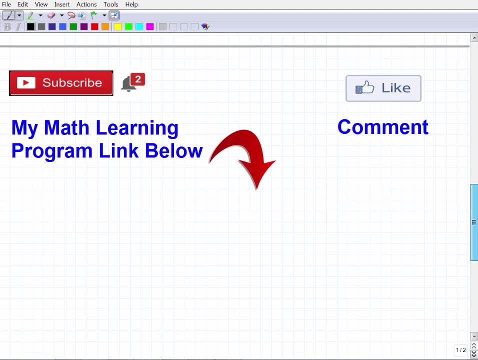 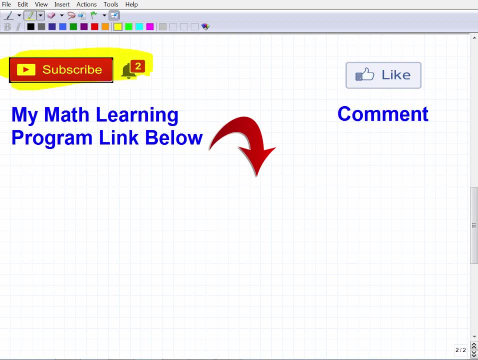 I actually have plenty more examples in a lot of my videos, so if you want to check those out, you can. So hopefully you'll consider subscribing. I also have a complete, many, many full, comprehensive math courses. I'll leave a link in the description of this video if you want to check those out. 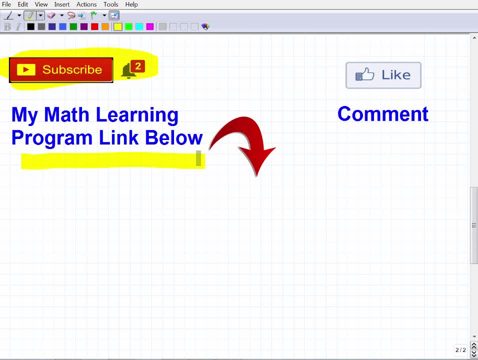 So if you're taking Algebra 1, I actually have complete, comprehensive Algebra 1 programs. I mean, I'm talking about full programs where I'm teaching complete lessons going over literally in my algebra courses, for example, several thousand problems. I'm showing you how to do them step by step. 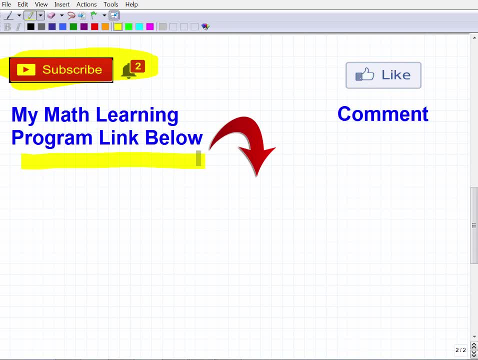 So it's a pretty. it's one of the most comprehensive courses. I think it's one of the best math learning programs out there. So if you like my teaching style and you really really want to learn from me, then check that out. 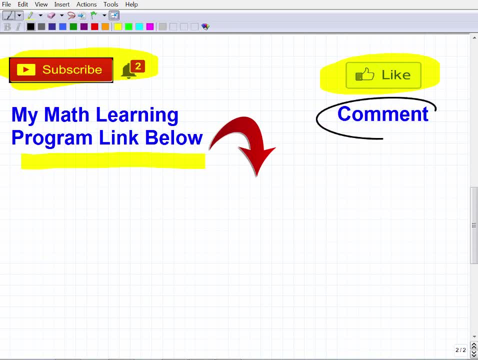 If you enjoyed this video. I definitely would appreciate a thumbs up and let me know what you think. You know how's math going for you? Maybe you have more questions if you're confused about something. I try to read as many comments as possible, but it lets me know how I'm doing. 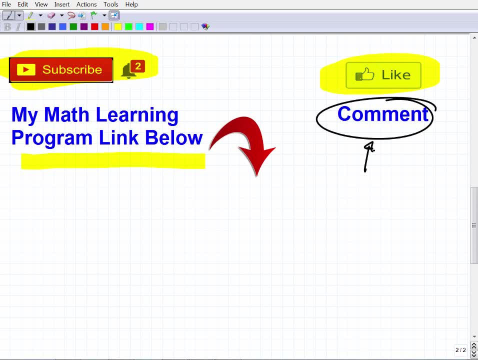 It also gives me ideas for future videos. But, with that being said, I definitely appreciate your time. I wish you all the best in your mathematics class And have a great day. 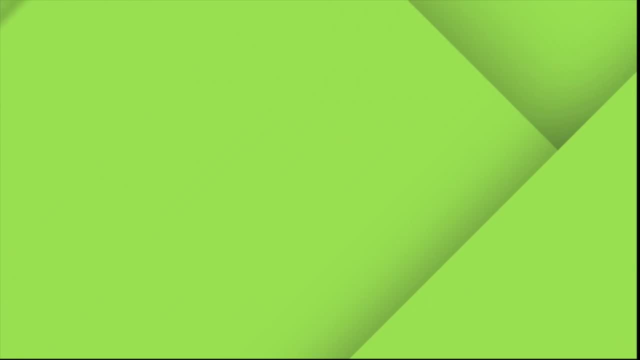 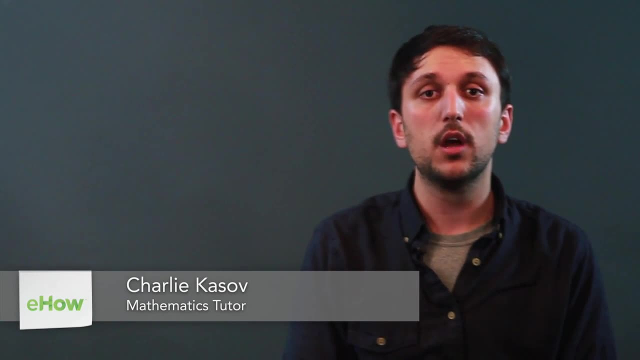 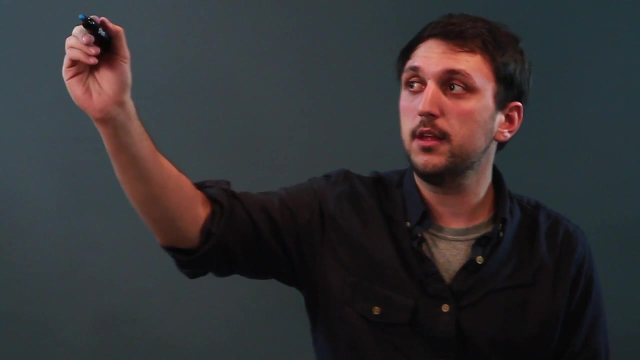 Hi, I'm Charlie Kasov. I'm a math teacher, and today we're going to learn how to find the volume of a cylinder using the diameter. So first let's explain what the volume of a cylinder equation is, and that is: volume equals pi r squared h. 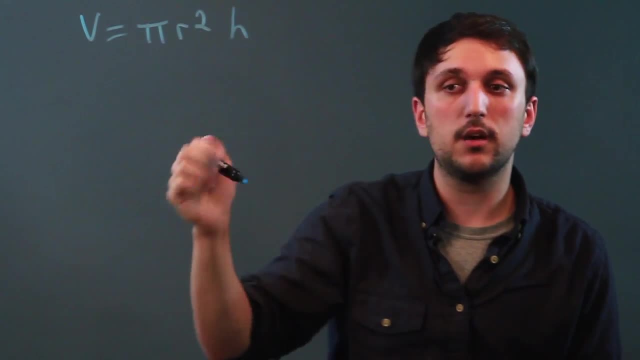 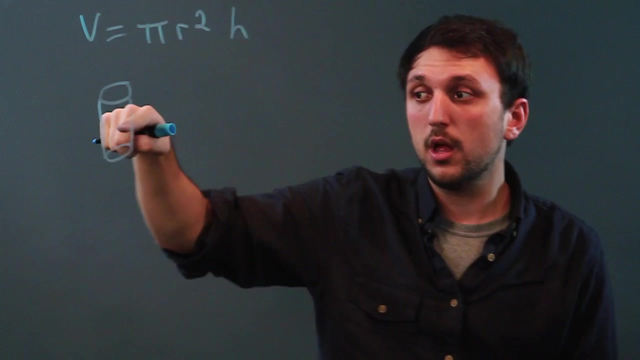 Now you may recognize pi r squared. That's the area of a circle. When you have a cylinder, you want to think of a cylinder as a bunch of circles stacked on top of each other. Now, if the area of each circle is pi r squared, then you just multiply by the height and that's how many circles. 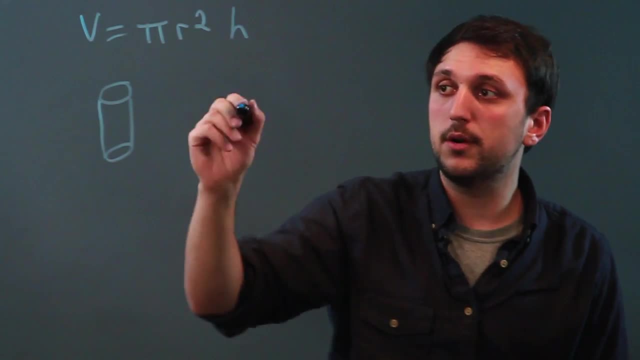 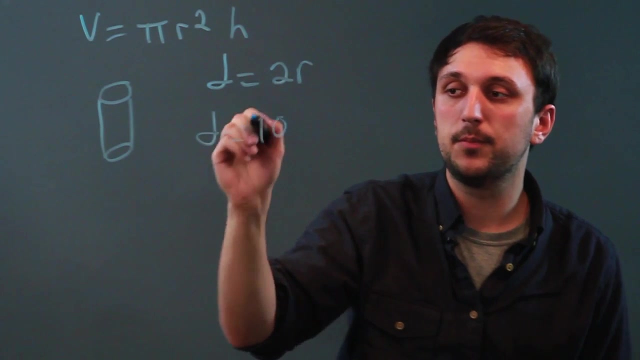 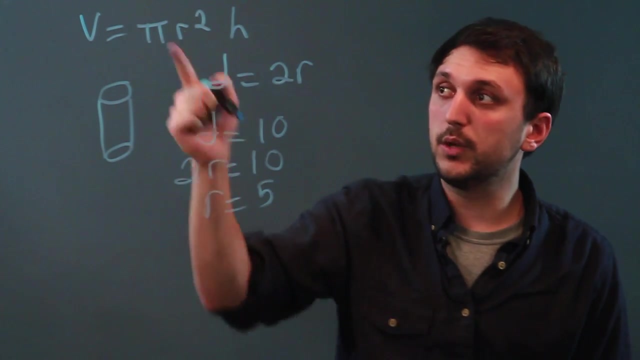 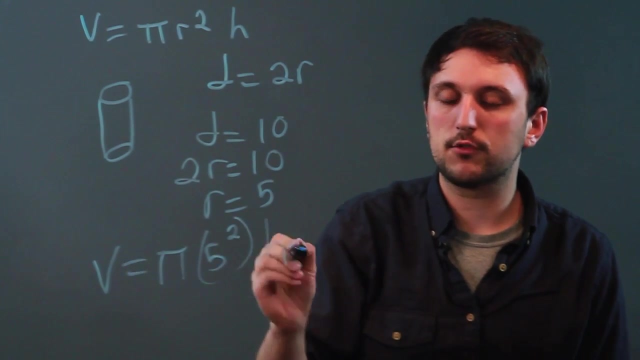 So the problem is: where is the diameter? Well, the diameter is 2r. So let's say we have a diameter of 10.. That means 2r equals 10, and that would mean that r equals 5.. So we can plug it into the equation: v equals pi 5 squared h. 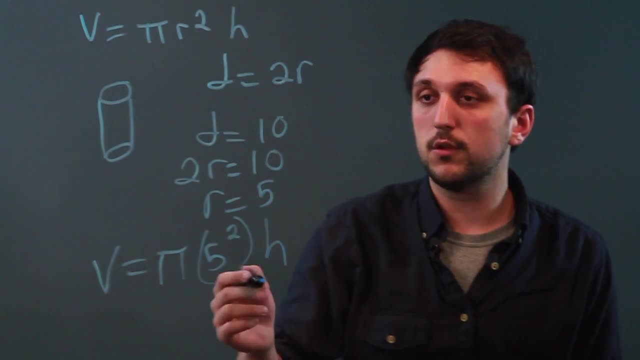 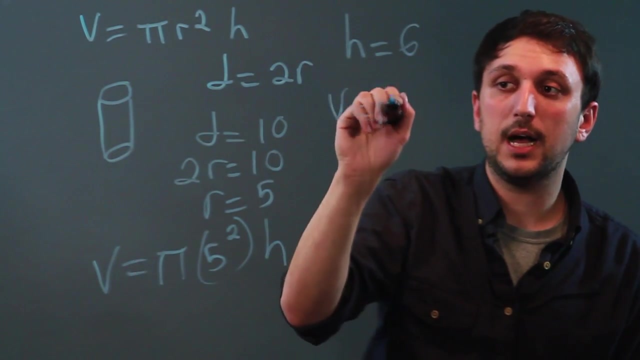 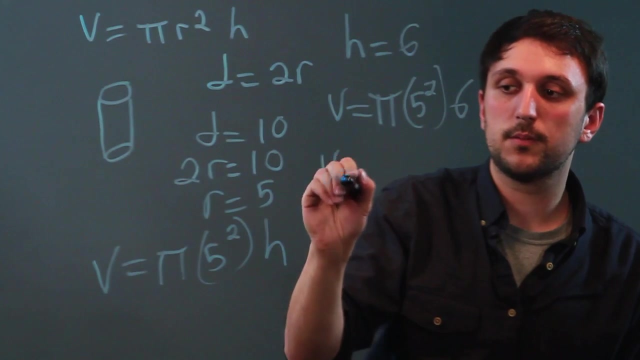 Well, where's our h? We would still need an h. So let's make h equal to 6.. So now we can say: v equals pi 5 squared times 6.. So 5 squared is 25.. So 25 pi times 6.. 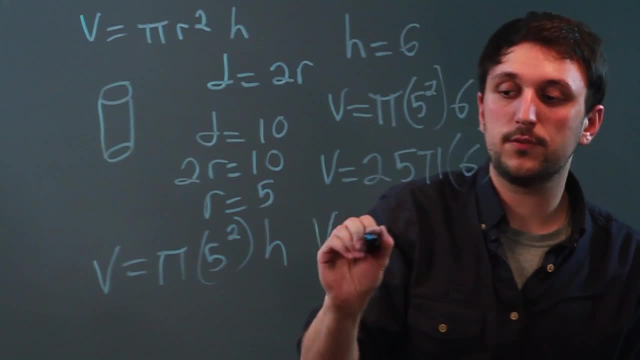 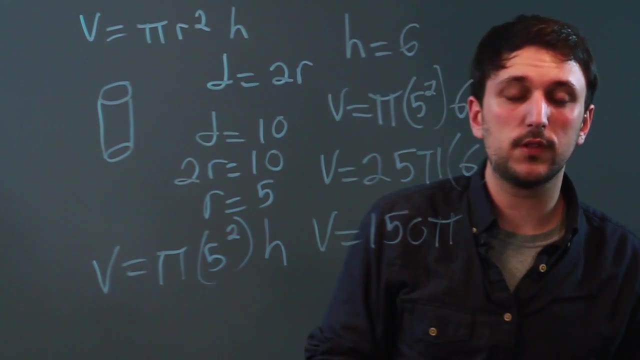 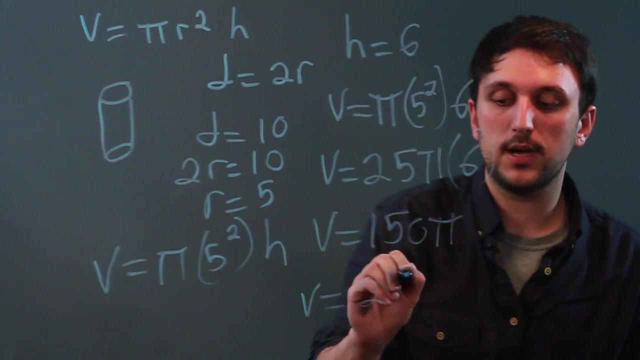 Which is 25 times 6, is 150. So the volume is 150 pi. So in order to find the volume of a cylinder using the diameter, you would need the height. Otherwise, if we didn't know the height, we would have to call it: volume equals 25 pi times h. 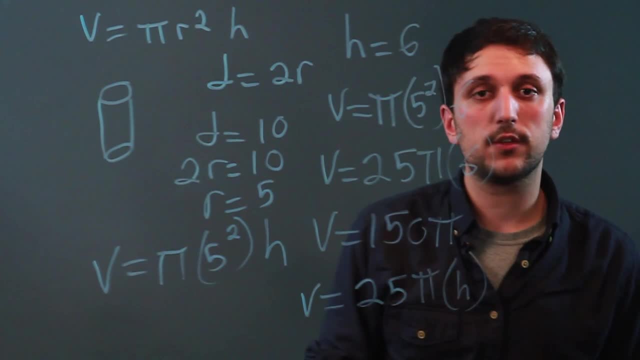 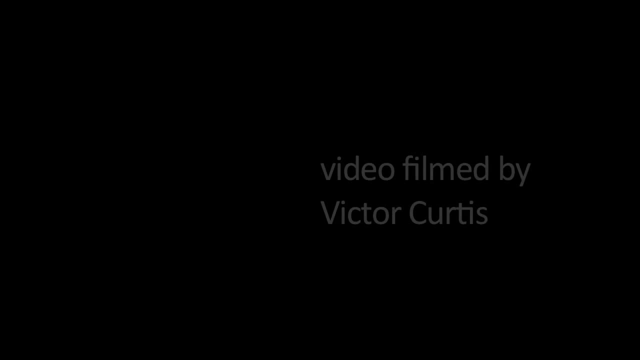 So I'm Charlie Kasov and you just learned how to find the volume of a cylinder using the diameter. Thanks, Thank you very much for watching. We'll see you next time. Bye, Bye, Bye, Bye, Bye, Bye.